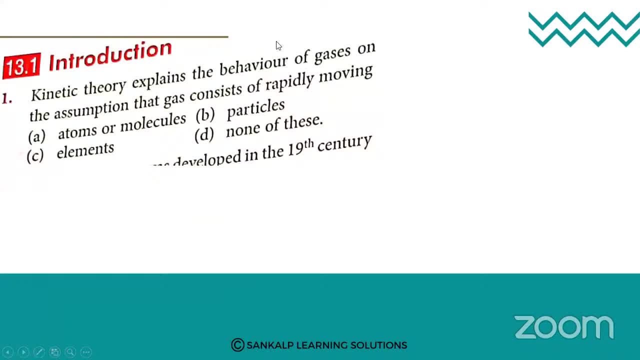 answer. please, in the chat box you tell the answers. Yes, first question: Kinetic theory explains the behavior of gases on the assumption that gas consists of rapidly moving. Yes, according to kinetic theory of assumptions, kinetic theory of gases, the gas consists of rapidly. 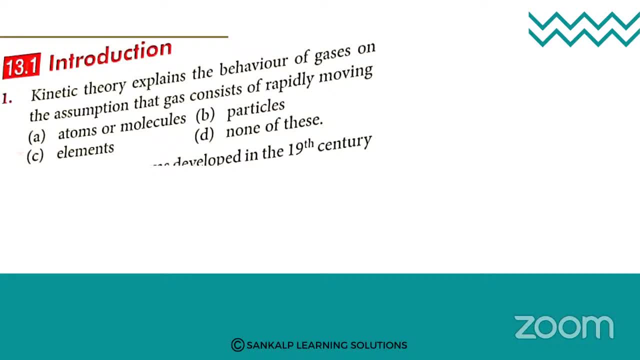 moving items or molecules, particles, elements? none of this. Yes, what will be moving according to the kinetic theory of gases? Yes, Madan Navya Sana. What will be moving? So this is the basic question, based on the kinetic theory of gases, assumptions. 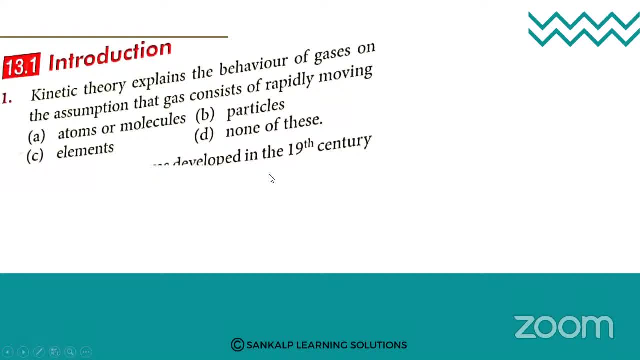 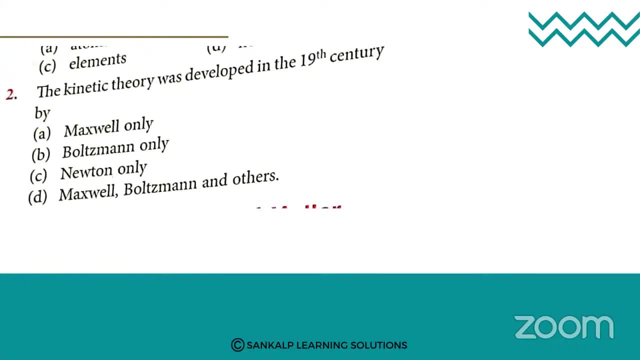 Based on the theory that is, the atoms or the molecules will be moving. Go for the next question C. The kinetic theory was developed in the 90th century by. Yes, who proposed this kinetic theory? Maxwell Boltzmann, Newton, Maxwell Boltzmann and others. Yes, So the. 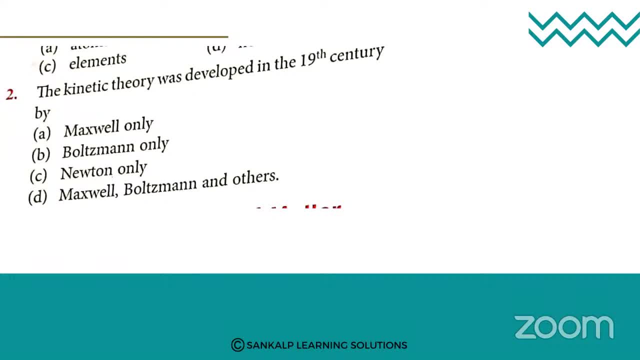 second question that was asked more by N Bukovic Kuffman. The third question that was asked most often and most popularly were: fewer bugs and more nasions Medium size and very a few little bugs. Topological topic is magnetic, Yes, and 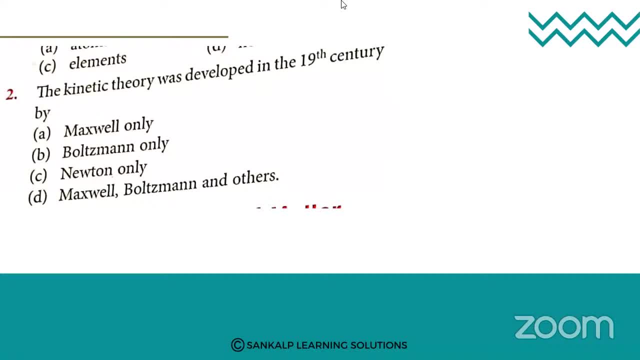 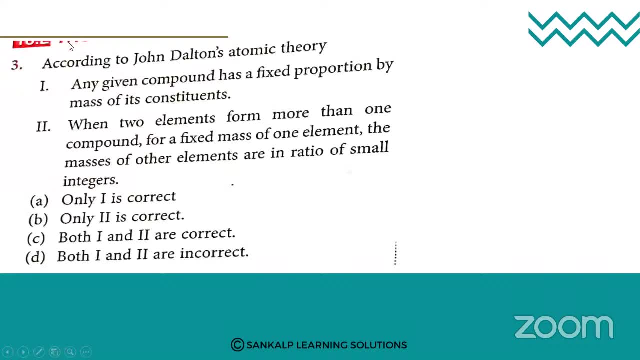 see, the kinetic theory was proposed by boldsman maxwell. okay, the next question. according to john dalton's atomic theory, any given compound has a fixed proportion of mass of its constituents when two elements form more than one compound. for a fixed mass of one element, the masses of 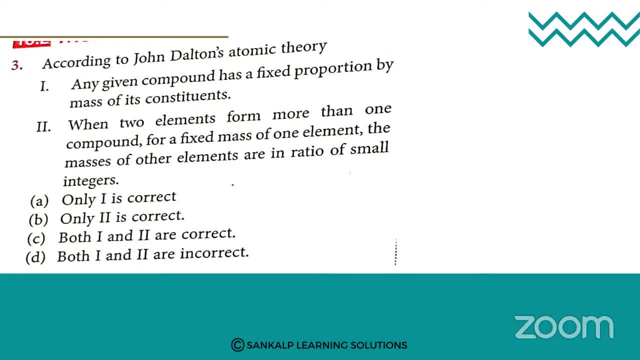 other elements are in the ratio, are in the ratio of small integers. so here both the statements, so two statements. they have given whether both the statements are true, only one statement is true or both are not true, that you need to answer here so you can see that is first what they are saying. any given compound has a fixed proportion of mass of its 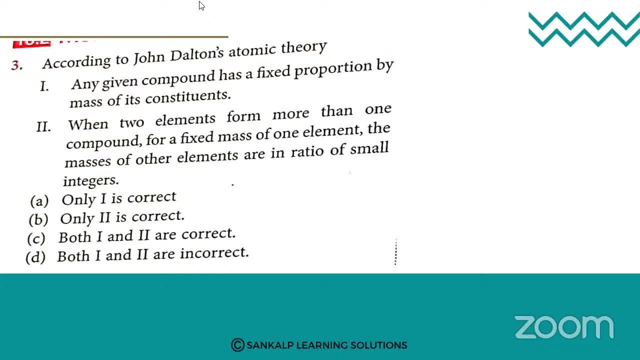 constituents. so this is true or no? option c, that is. both the statements are correct. yes, option c is correct, that is, any compound has the fixed proportion by mass of its constituents. but then when two elements form more than one compound for a fixed mass of one element, 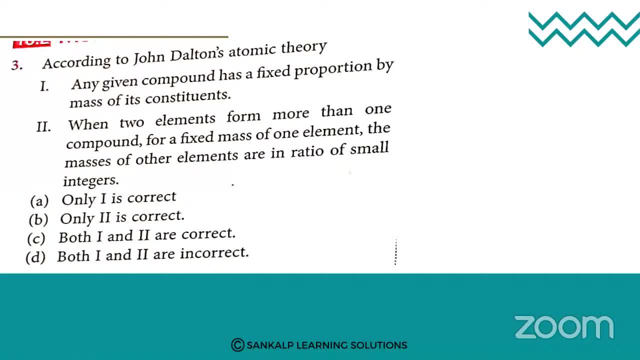 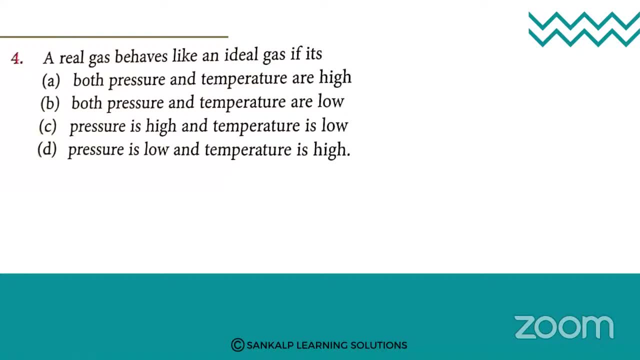 the masses of the other element are in the ratio of the small integers. both the statements are true. go for the next question c: a real gas. a real gas behaves like an ideal gas if it's. both pressure and temperature are high, both pressure and temperature are low. pressure is high and temperature is low. pressure is low. 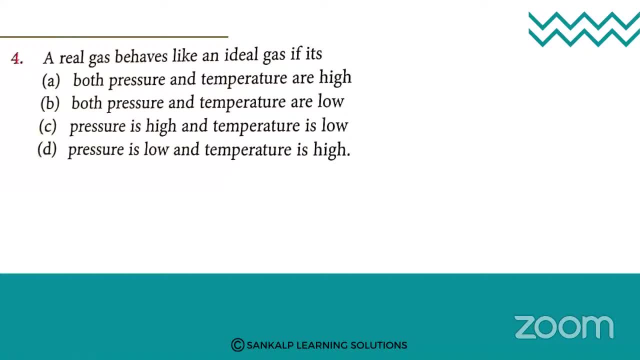 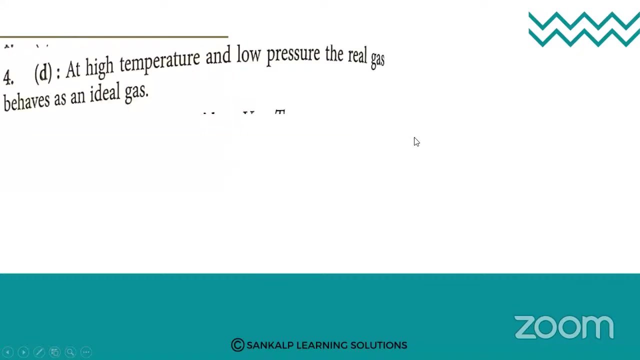 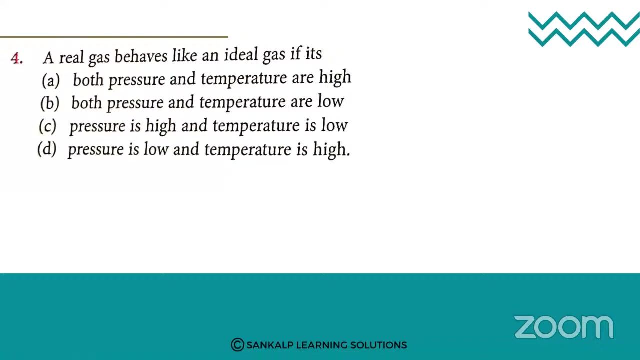 and temperature is high, you see, for the ideal gas. if you are saying it is ideal gas, the gaseous must obey that is, at high temperature and the pressure must be low, then you can call the gases as the ideal gases if you maintain that condition. it. 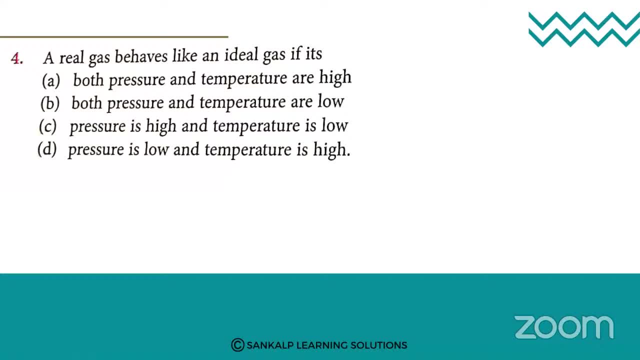 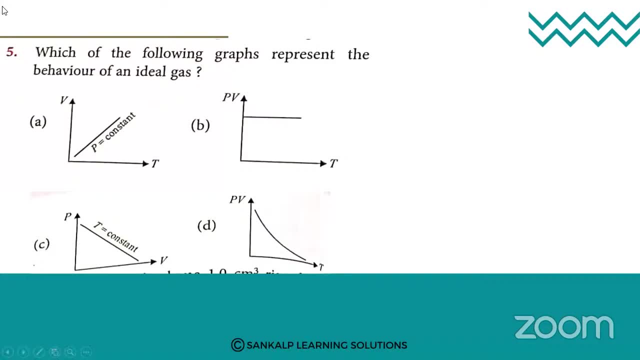 behaves like a real gas, is like a ideal gas. okay, next, which of the following graphs represent the behavior of an ideal gas? so, with respect to the ideal gas, the pressure b pressure, temperature and volume axis, with respect to three quantities. they are giving that graph. so which is which you can, which will describe the ideal gas? 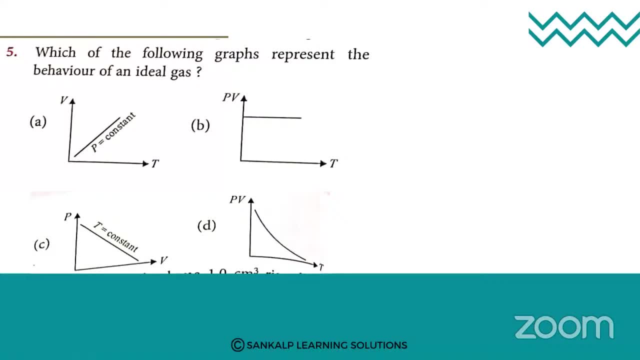 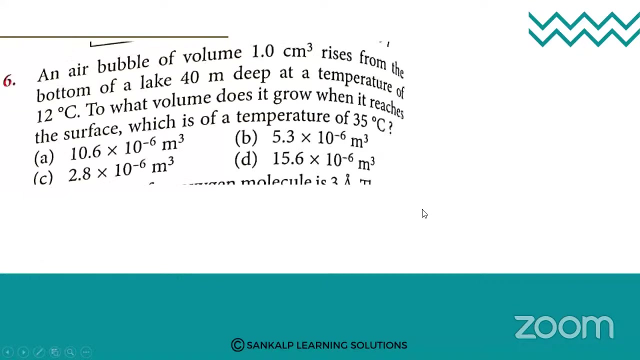 the one that will be describing it as a all-estone- we call it a high-tech élixir- is which the graph will describe so you can history. that is the first graph. so, according to the first graph, that is, volume and temperature. yes, which graph will describe so you can see here. that is the first graph. so 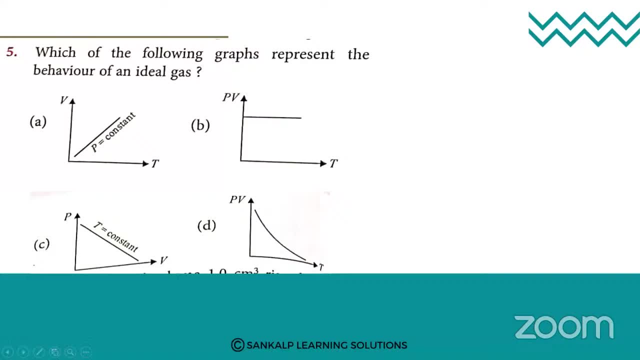 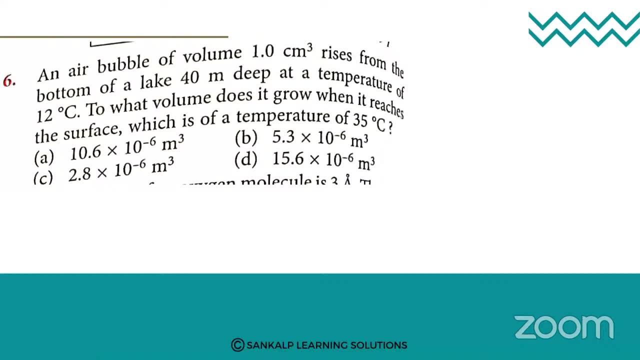 according to the first graph, that is, volume and temperature, energy you variables, and the pressure is remaining constant. the next question, so numerical based it, is an air bubble of volume. one centimeter cube rises from the bottom of a lake 40 meter deep at a temperature of 12 degrees celsius. to what volume does it grow when it reaches the surface? which? 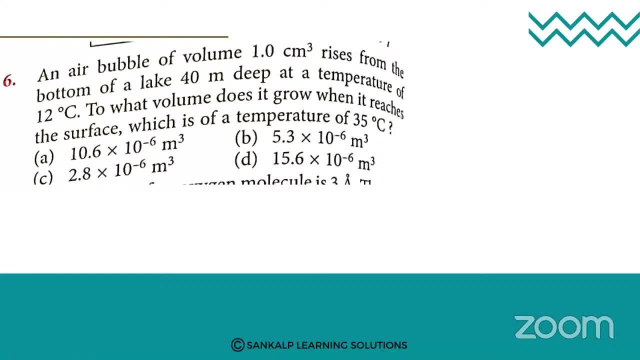 is of the temperature of 35 degrees celsius. so the two temperature value is given, then the height and the volume value they have given. so they are asking: when you are increasing the temperature, what will be the increase in the volume? copy down the question, we will see how to solve it. 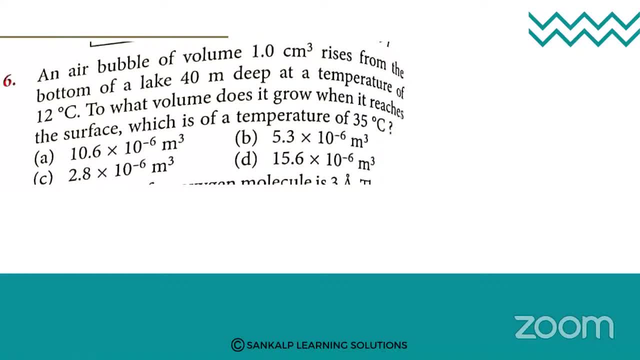 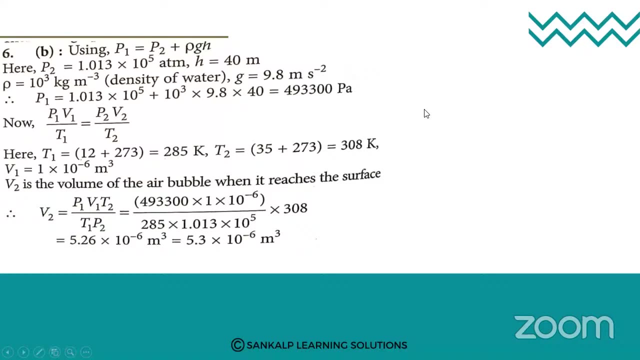 it's completed. okay. so see here, students. that is, the pressure is equal to p1, is equal to p2 plus rho gh. so p2 is the atmospheric pressure. otherwise you can consider it as p naught also. so p naught also you can denote. you can denote it as p2. 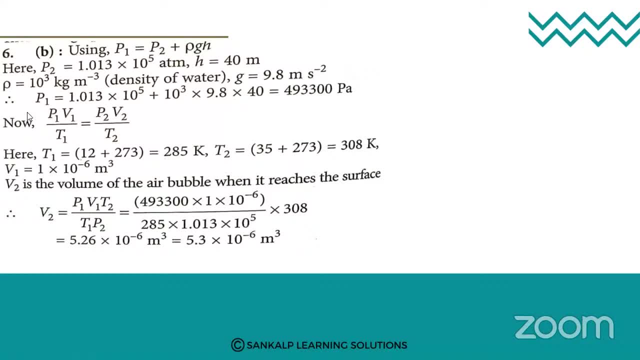 So that is describing the atmospheric pressure. okay, So that is given by the equation. You can write it as P1 plus P0.. P1 is equal to P0 plus rho gh, where your P0 is atmospheric pressure and its value is taken as 1.013 into 10 raised to 5 atmosphere. 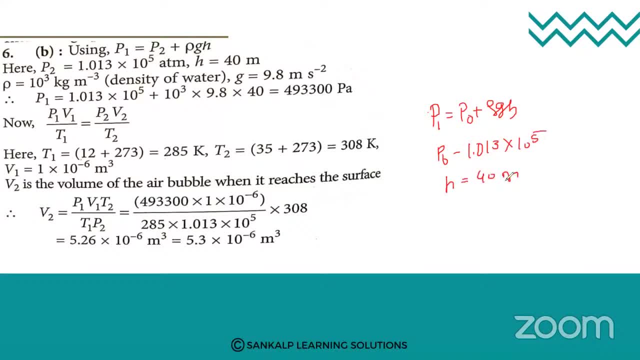 And the height value is given. The height value is given as 40 meter, okay. Acceleration due to gravity is mentioned as 9.8 and the density is given as 10, raised to 3 kg per meter cube. okay, So therefore, P1- V1 divided by T1 is equal to P2- V2 divided by T2.. 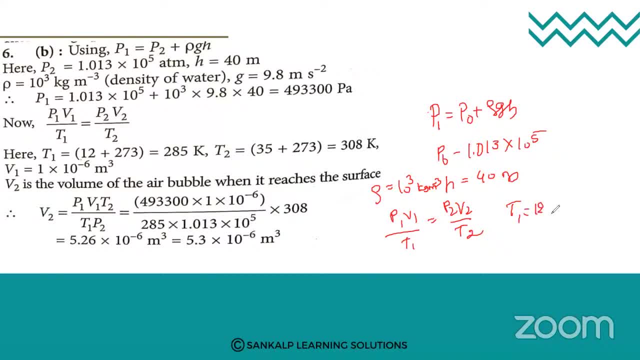 So here the temperature: T1 is how much That is. it is given as 12 degree Celsius. converted in terms of degree Celsius Kelvin, that is plus 273.. So 273 plus 12 is nothing, but what 285 Kelvin, Similarly, T2 is equal to you can do: T2 will be 35 plus 273.. 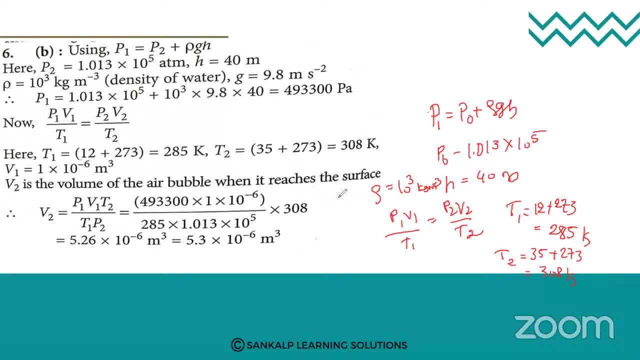 How much it will be. It will be 308 Kelvin. okay, So first initial volume is given in the question. So initial volume is given as 10 raised to minus 6 per meter cube. So what will be V2?? 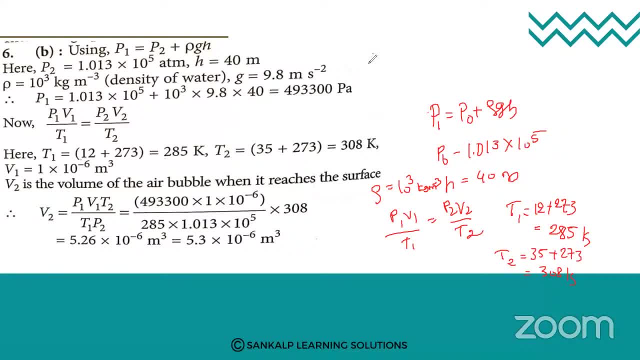 So according to the ideal gas equation, So we have the equation: P1, V1 is equal by T1 is equal to P2, V2 divided by T2.. We require V2.. Therefore the other terms you just transfer here, that is, P1, V1, T2 divided by T1 into P2.. 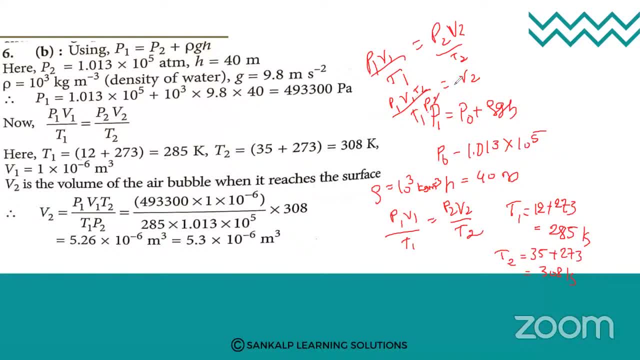 So all the values you know. just substitute the values and simplify, you will get. V2 is equal to 5.3 into 10 raised to minus 6.. Yes, see the calculation. if you have any doubt, you can ask. So V1 is 1 into 10 raised to minus 6, P1 into T2.. 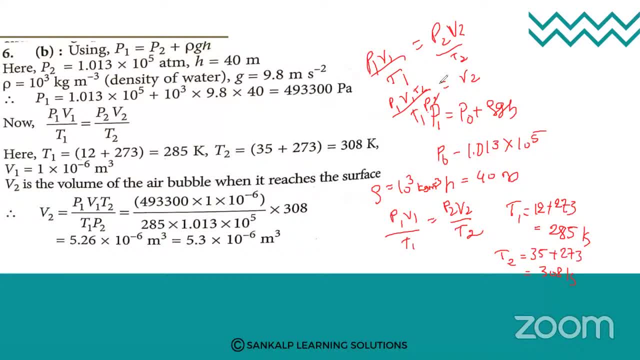 So temperature is 308 T2 and in the denominator we have 285 into P2.. So multiply and divide the answers, you will get it as So 5.3 into 10, raised to minus 3 meter cube: Yes, completed students. 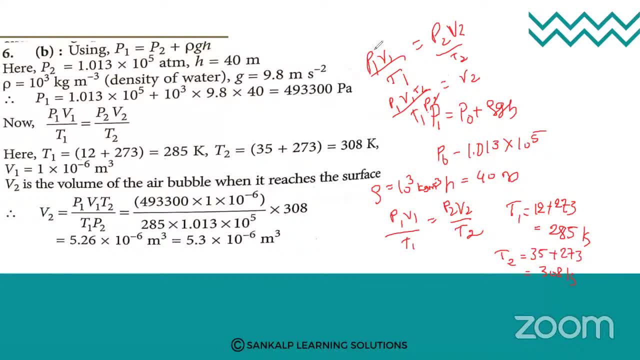 Yes, completed, students. We are going for the next question. Next question is the diameter of an oxygen molecule. Next question is the diameter of an oxygen molecule. Next question is the diameter of an oxygen molecule. The diameter of an oxygen molecule is given as 3 angstrom. 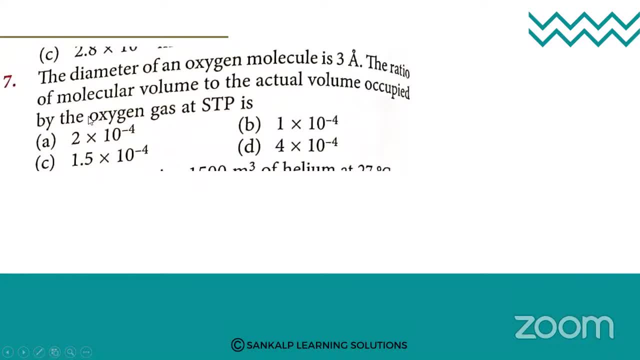 So the diameter of oxygen molecule is given as 3 angstrom. The ratio of molecular volume of the actual volume occupied by the oxygen gas at STP is: See what they are saying here. The diameter of an oxygen molecule is 3 angstrom. 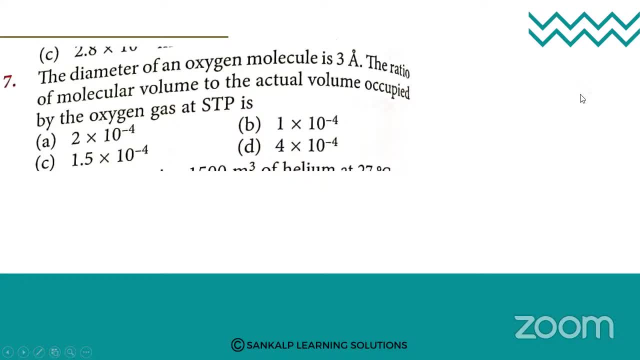 So its diameter is given as how much. It is given as 3 angstrom. Okay, So the diameter is 3 angstrom The ratio of the molecular volume. So the ratio of the molecular volume to the actual volume. 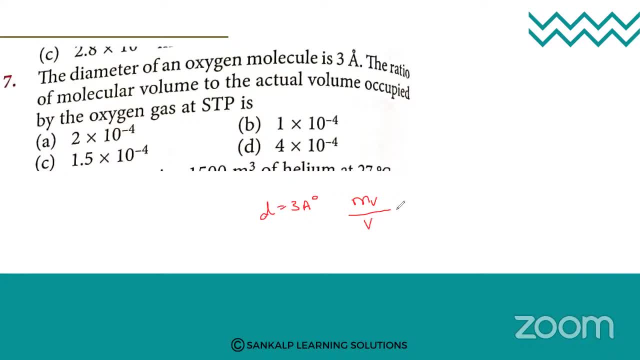 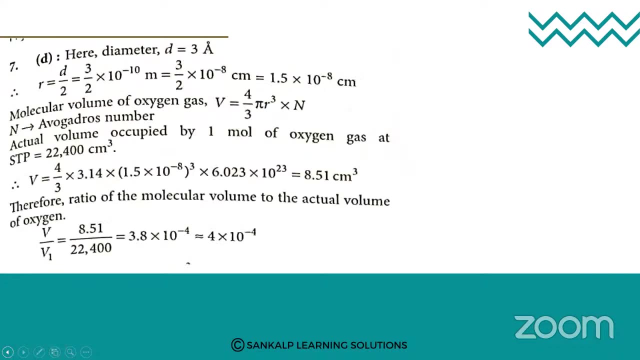 So to the actual volume occupied by the oxygen at STP is given by: So at STP, what is the value that you need to calculate? Let's see So here. whatever the diameter is given, take the radius of that that is divided by 2, you will get. 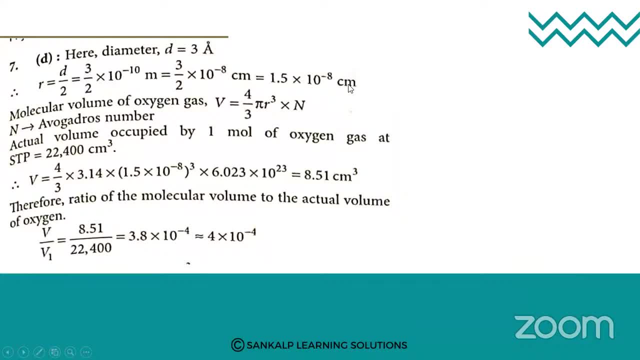 So it is divided by 2.. So it is divided by 2 or 1.5 into 10, raised to minus 8 centimeter. Then molecular volume of the oxygen is taken as 4 by 3 pi r cube into n. 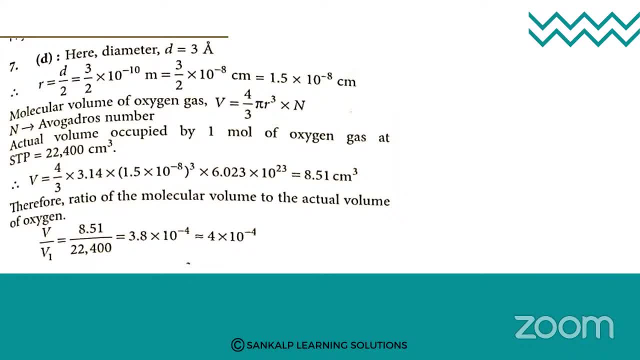 Okay, n is the Avagadro number. Next, actual volume occupied by 1 mole of oxygen gas at STP is: So it is a standard value at STP. What is the volume occupied by the oxygen gas? It is 22,400 centimeters. 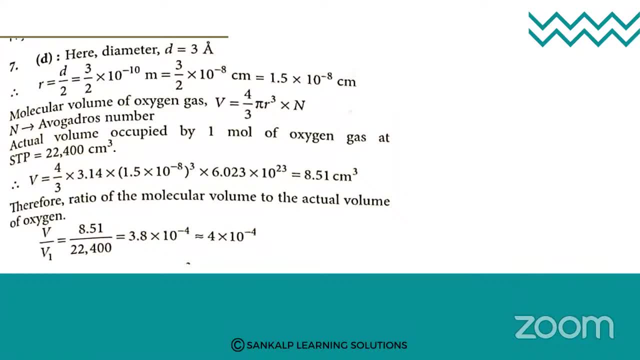 centimeter cube at stp, the volume of the oxygen is this constant value? okay, so 22,400 centimeter cube. so now we are calculating v is equal to. so when you are calculating v is equal to, just substitute here v is equal to n. by the formula it is 4 by 3. pi r cube into n, correct? so therefore 4 by 3 keep. 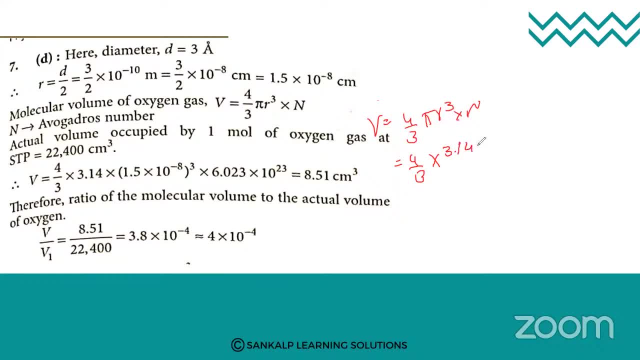 it as it is the one point. this pi is 3.14 into r, value is 1.5 into 10. raise to minus 8. it's cube, okay. the next avagadro number. the avagadro number is 6.023 into 10 to the power of 23. so if you 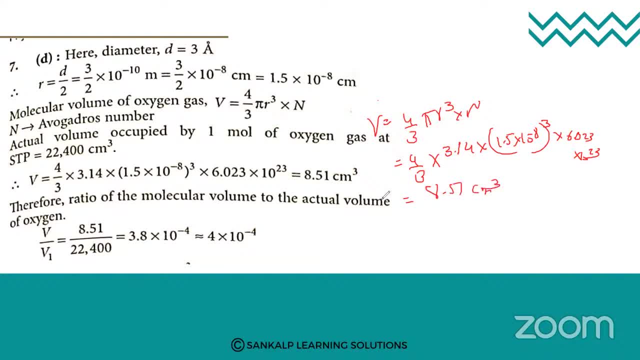 simplify this, you will get it as 8.51 centimeter cube. this is the volume. okay, so what they're asking? the ratio of the molecular volume to the actual volume. so what is the molecular volume volume here, students? so molecular volume, just now you have calculated: it is 8.51 divided by what is the actual volume, it is 22,400. so if you simplify, 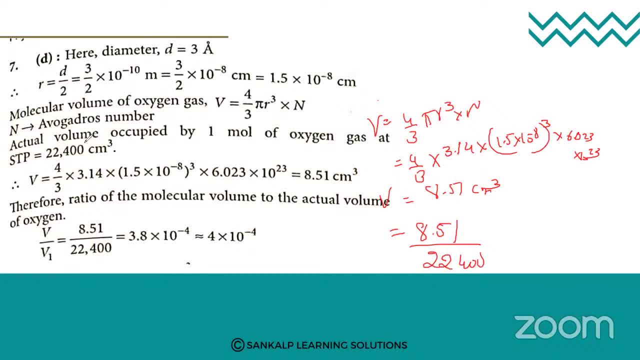 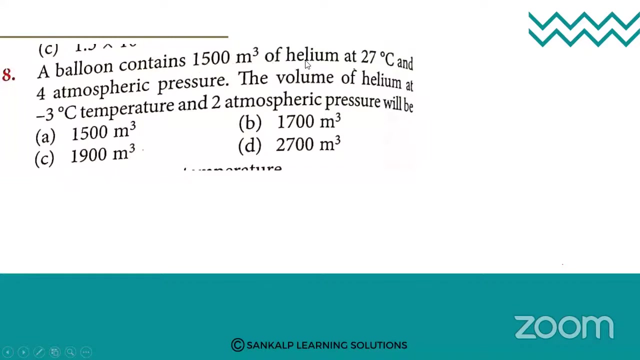 approximately. we'll get it as 4 into 10, raise to minus 4. you see the calculation. if any step you are not understanding, please ask with me. you, you, you do. you See the next question. A balloon contains 1500 meter cube of helium at 27 degree Celsius and 4 atmospheric pressure. 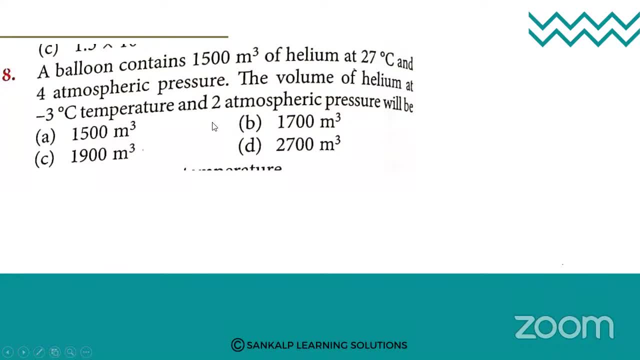 The volume of the helium at minus 3 degree Celsius temperature and 2 atmospheric pressure will be: A balloon contains 1500 meter cube of helium at 27 degree Celsius and 4 atmospheric pressure. So when the atmospheric pressure is 4 and the volume, the temperature, is 27 degree Celsius, the volume of the balloon is 1500. 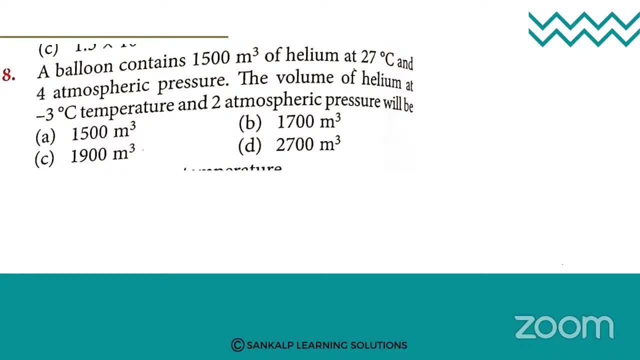 Next, what they are asking when the temperature is minus 3.. When the temperature is minus 3 degree Celsius and the atmospheric pressure is 2 atmospheric pressure, that time what will be the volume? So by taking the ratios of the volume, you can find out this one. 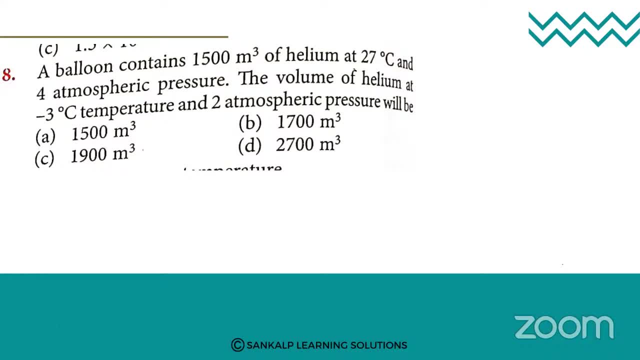 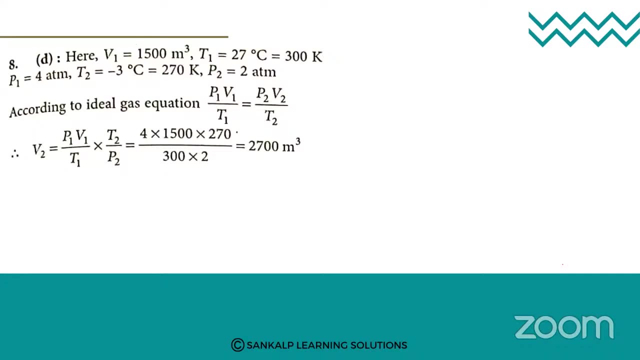 See This question is completed. What is the answer? Answer: See here Here: V1 is equal to 1500.. T1 is equal to 300 Kelvin, P1 is equal to 4 atmosphere And T2 is minus 3 degree Celsius. 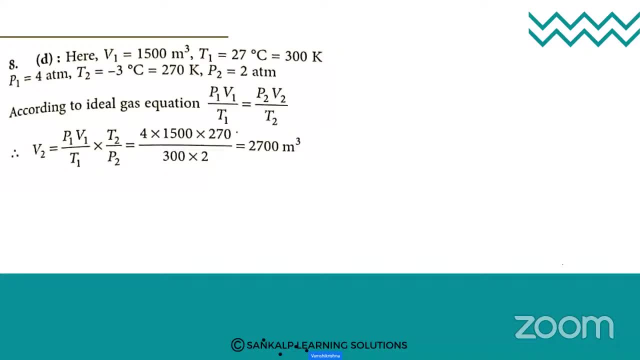 That is 270 Kelvin. So when P2 is 2 atmospheric pressure, what is the value of V2?? So simple question and simple solution. P1, V1 is by T1 is equal to P2, V2 by T2.. So substitute all the values. 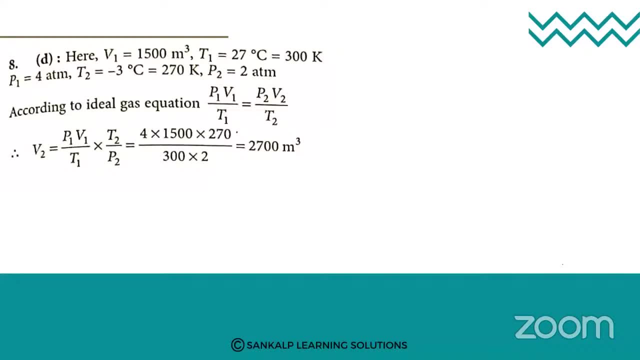 Only V2 is unknown to you. You can find out that very easily. Check whether You are getting it or no. You can check it. Yes, Everybody getting the answer. Please try: 2700 meter cube. Option D is the correct answer here. 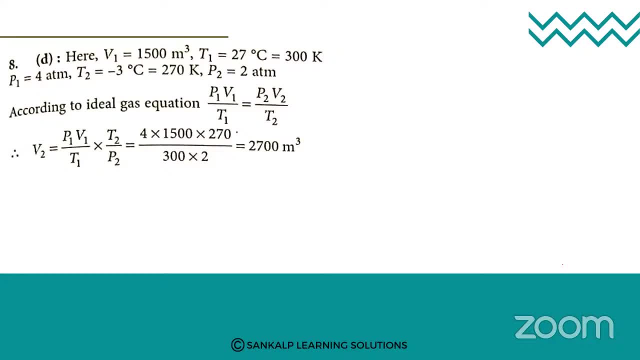 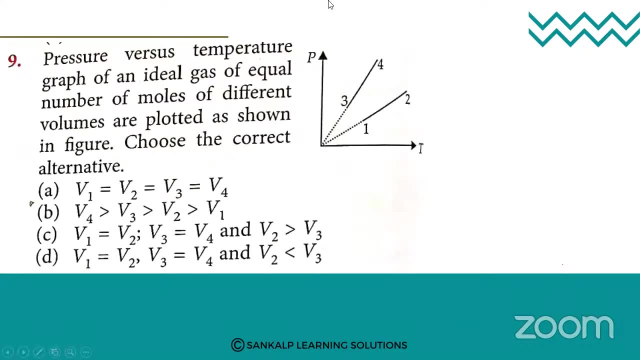 So you can get the answer if you are able to see the graph- pressure versus temperature graph for the ideal gas of equal number of moles of different volumes. So here the volume is, volumes are different are floated as shown in the figure. Choose the correct alternative. 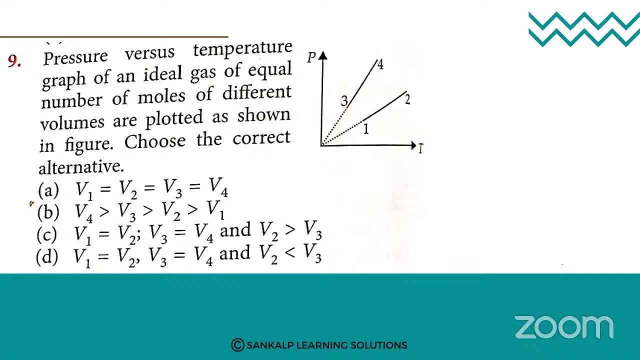 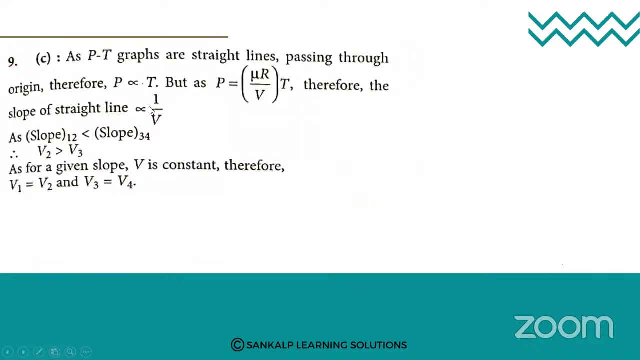 So here You are able to see 4 points in the graph: 1,, 2,, 3, 4.. So volume rate, volume relation they are asking in the given graph. Let's see here. That is according to the graph. 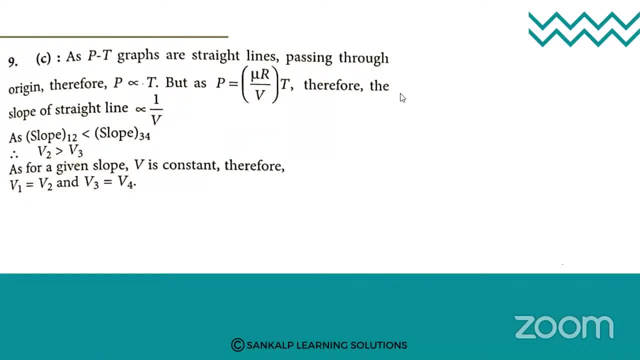 It is, pressure is directly proportional to temperature. Okay, So when pressure is directly proportional to temperature, Therefore the graph is a straight line, and when it is directly proportional, it is the inversely proportional to what will be. So pressure, temperature is directly proportional. 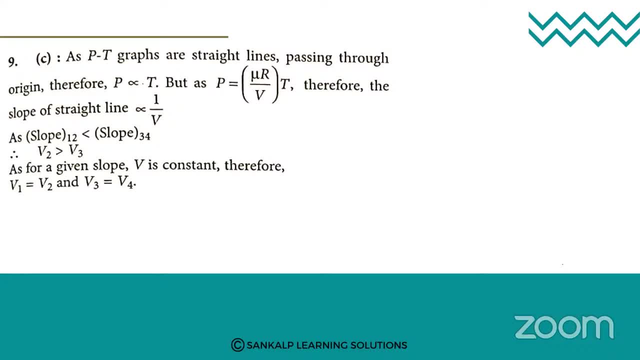 It doesn't mean a pressure is inversely proportional to volume, Correct. So therefore the slope of 1st and 2nd is less than the slope of 3 and 4.. You can see observe in this graph. So see: slope of 1st and 2nd is less than the slope of the 3rd and the 4th. 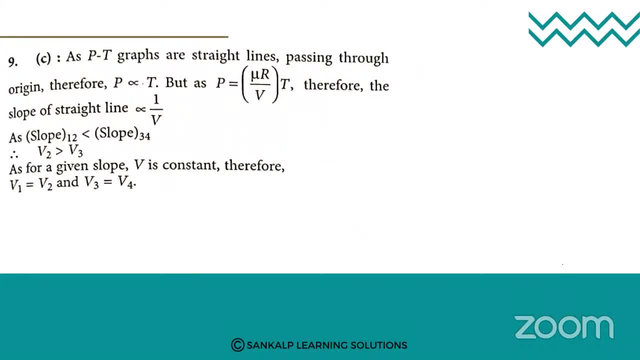 Correct, That is nothing but V2.. V2 is greater than V3.. Agree, Therefore V2 is greater than V3.. Means V3 value is lesser than the V2 value, So as the given slope V is constant. 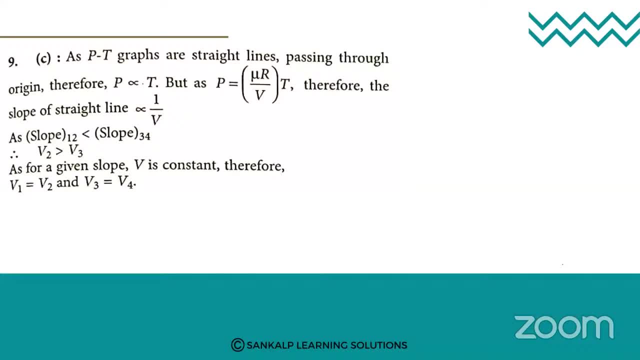 As the given slope, V is constant. Therefore V1 is equal to V2 and V3 is equal to V4. So if suppose if is equal to V4. If V is equal to V4, V is equal to V5.. 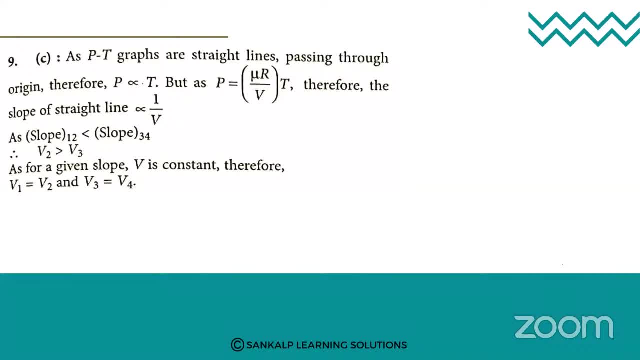 Then V3 is equal to V6.. So the answer is V2.. If V4 is equal to V6, it will be V3. So the answer is V6.. So that is V3.. So the answer is V5. 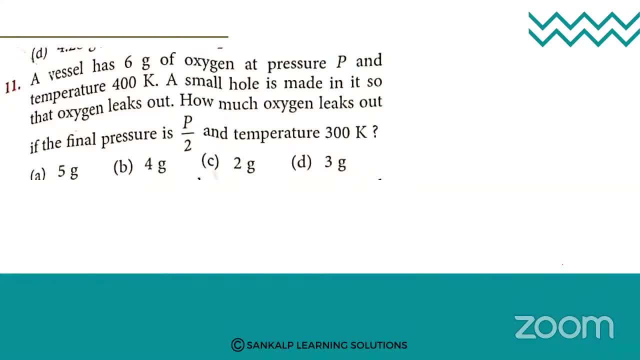 So that is V4.. So here you can see, V4 is similar to the point, So it is equal to V6.. Right? So question is: is what a vessel has? 6 gram of oxygen at pressure P and temperature 400 Kelvin? 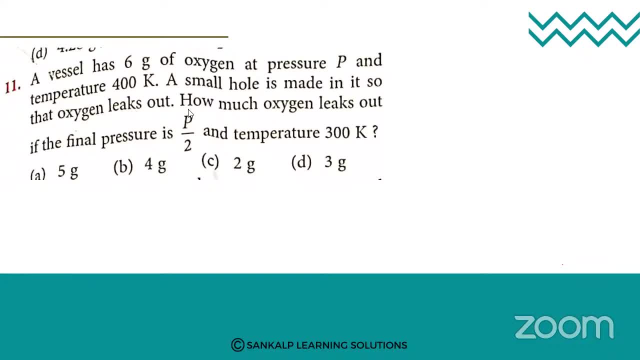 A small hole is made in it so that oxygen leaks out. How much oxygen leaks out if the final pressure is P by 2 and the temperature is 300 Kelvin? So pressure is reducing from P to P by 2.. Temperature is from 400 to 300 Kelvin. 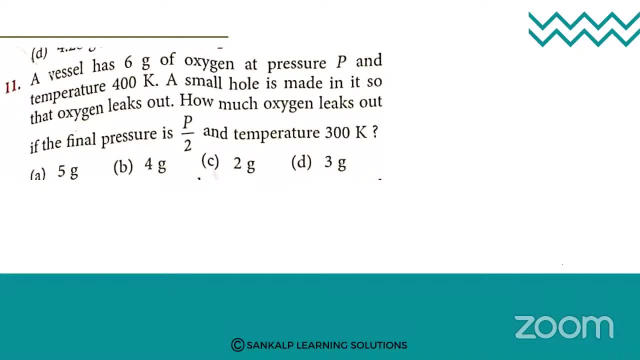 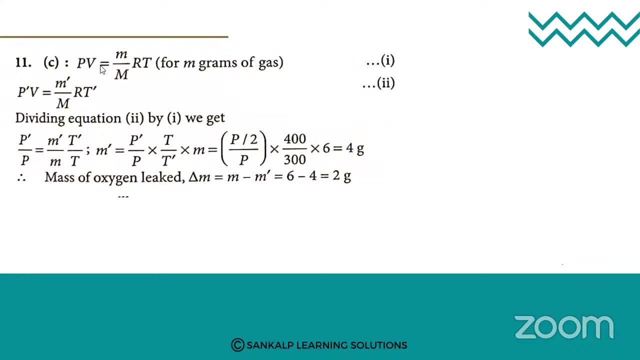 What happens to the mass? First it was 6 gram, Next what will be the mass? So think on it, students, how to do it. Yes, that is. PV is equal to m upon mRT for m gram of mass. 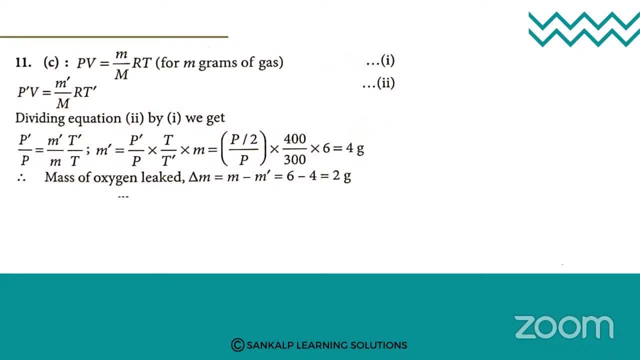 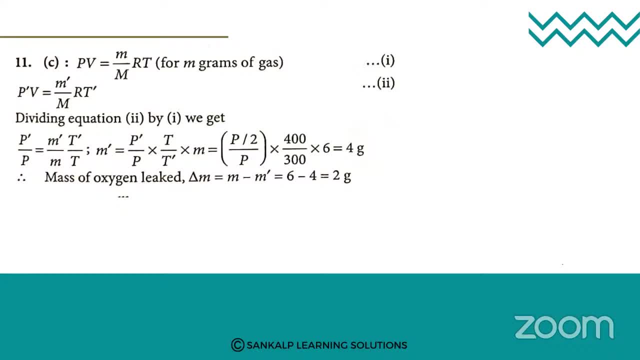 Dividing equation 2 by 1. What we will get, That is, P dash by P is equal to m, dash by m. mRT will get cancelled, So we are having the ratio of only pressure mass and the temperature. Okay, 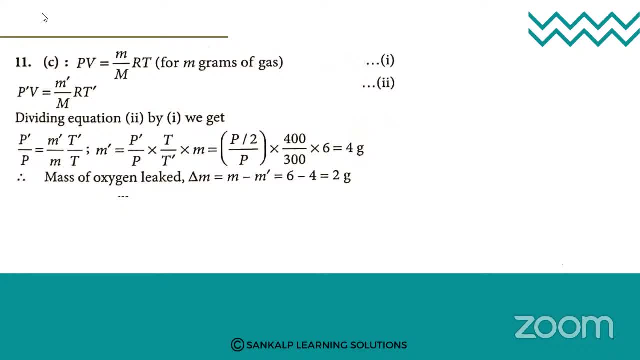 So pressure is increasing, P is increasing. Pressure is increasing, P by 2. Temperature: 400 to 300 it is coming. So now mass is coming out to be 4 gram. So the mass of the oxygen is leaked out. 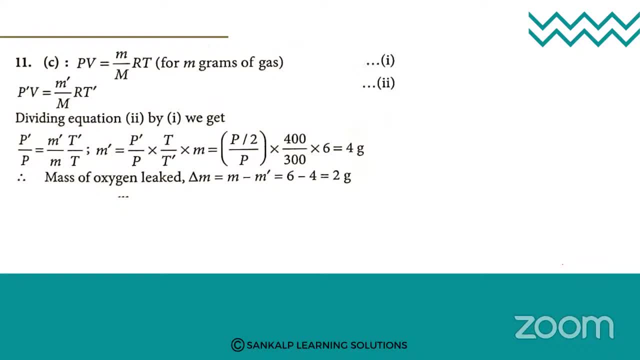 So we have to find out the difference in the mass. The initial mass was 6 minus. now, after that leakage, it is minus 4, which is equal to 2 gram of mass is remaining. So therefore, 2 gram is the answer. 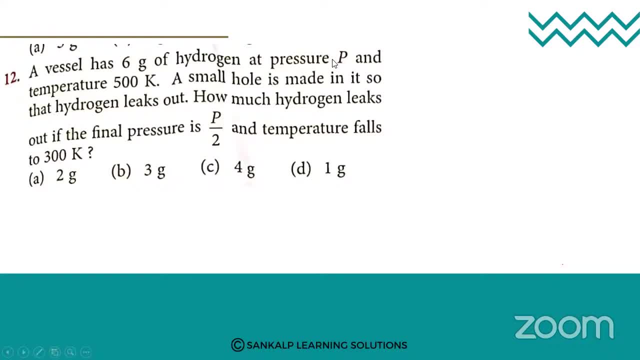 Next question: A vessel has 6 gram of oxygen hydrogen at pressure P and temperature 500 Kelvin. Okay, So same question. Little quantities are different. Please try this, students. Pressure is changing from P to P by 2. Temperature is from 500 to 600. 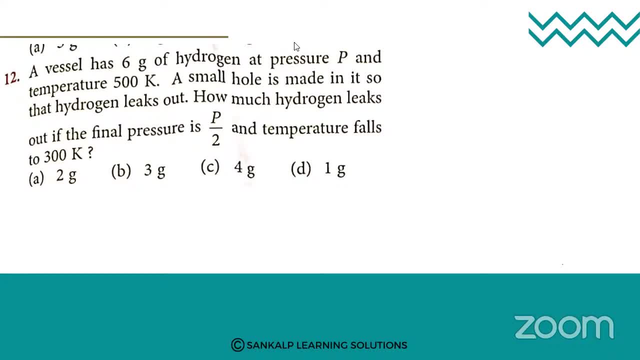 Sorry, 300.. Check what will be the mass Now. we have a full mass, We have 2.. We have 4.. The mass is being reduced by 2.. We have 1.. It will be more than 2.. 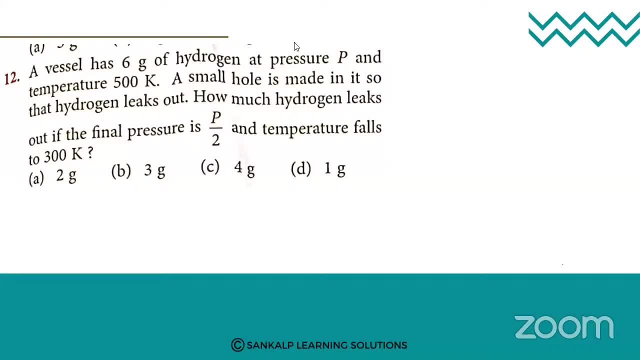 The mass is being reduced by 2. It will be more than 1. 1. 1. 1., 1., 1. 2., 1., 2. 1., 2., 1. 1.. 1., 2., 2., 1., 2., 1., 1., 2.. We will see 3., 3., 3., 2., 2., 8., 9., 6.. 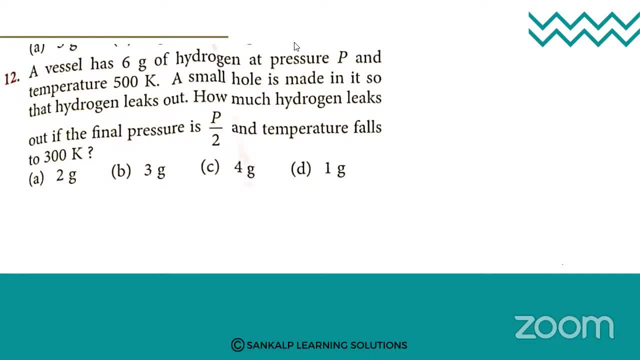 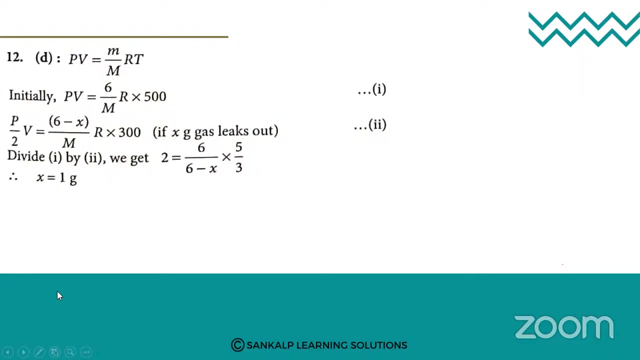 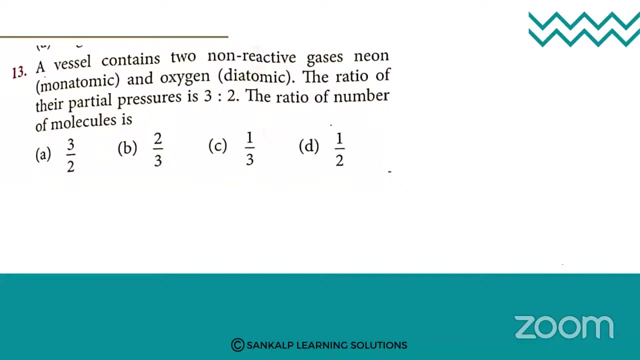 7., 5., 6., 8., 9., 9., 9., 10., 11. you, yes. what is the answer? everybody is getting d. okay, yes, d is the correct answer, so go for the next question, students. a vessel contains two non-reactive gases, that is, neon and the oxygen. 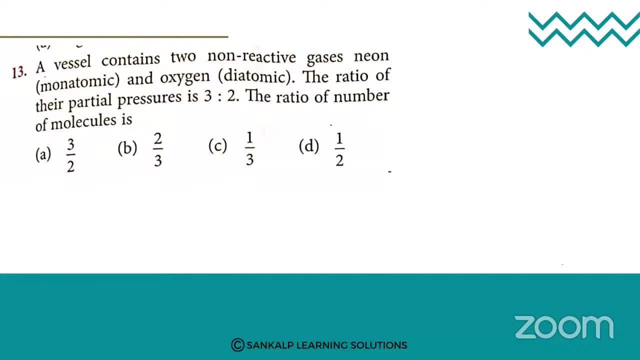 so both are mono, one is monotonic and one is the diatomic. the ratio of their party partial pressure is three is to two, so the ratio of their partial pressure is three is to two. the ratio of number of molecules is, so the ratio of their partial 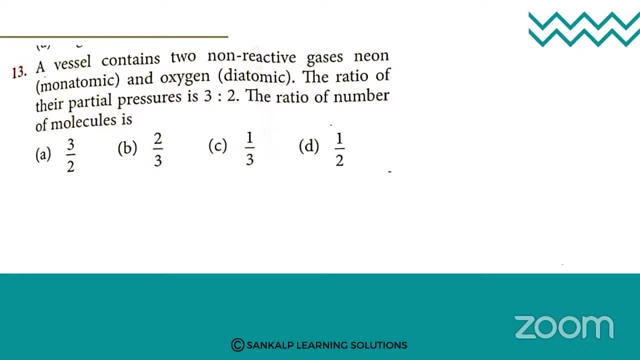 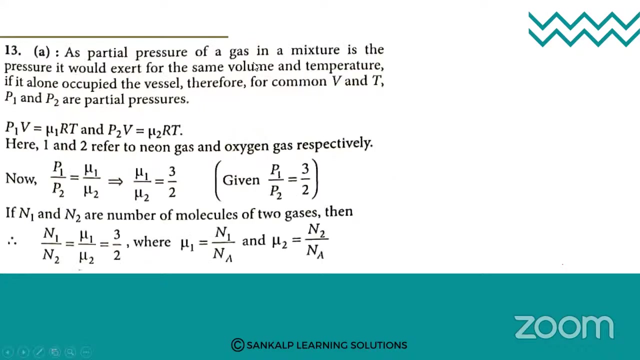 pressure is. three is to two. ratio of number of molecules: yes, see how to do it. so, as the partial pressure is what it is, the mixture of the two different gases it is given. so therefore, here, p1 v1 is equal to mu1 rt and p2 is equal to mu2 rt. so if you take the ratio, 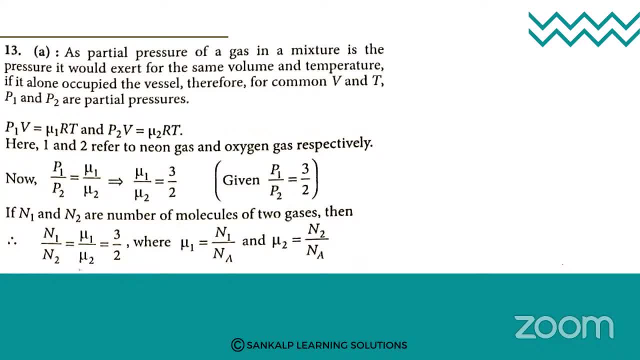 rt term and the volume term will get cancelled. so next, the mu1 by mu2 ratio is given as 3 by 2, so therefore p1 by p2 ratio will be 3 by 2, and n1 and n2 are the number of molecules of the two. 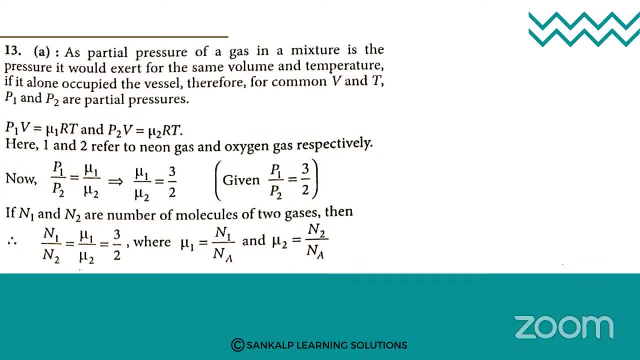 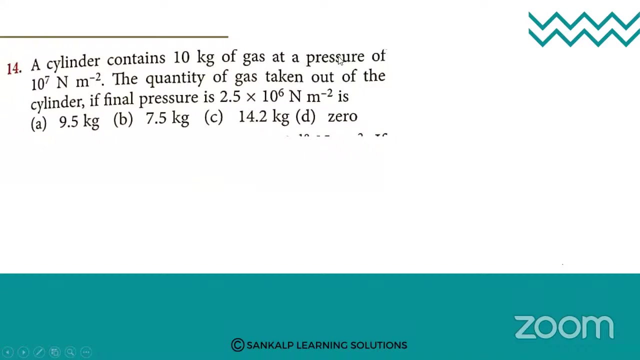 gases. then n1 by n2 is equal to mu1 by mu2 is equal to. it will be 3 by 2. yes, so where mu1 and mu2. what it is, it is written there. so go for the next question, students. a cylinder contains 10 gram of gas at a pressure of 10. 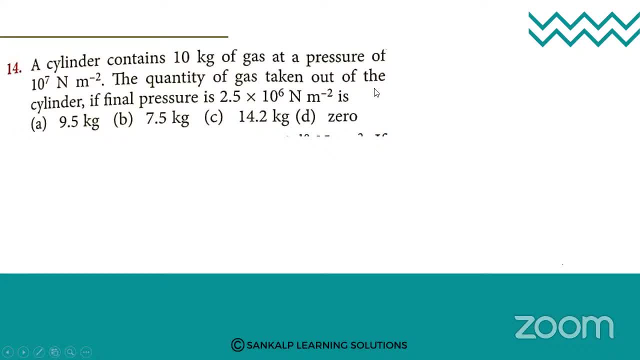 is to 7 newton per meter square. the quantity of gas taken out of the cylinder. if the final pressure is 2.5 into 10, is to 6 newton per meter square. see cylinder contains 10 gram of gas. at a pressure of 10 is to 7 newton per meter square the quantity of gas. 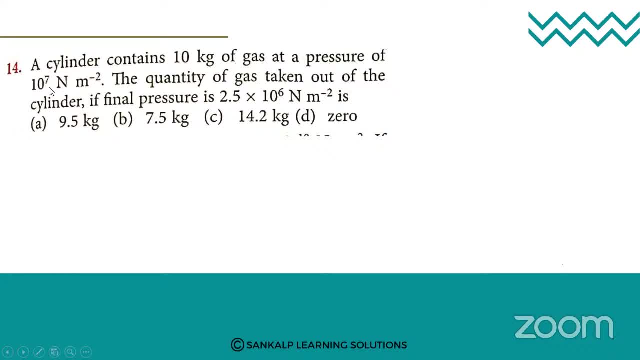 10 gram, 10 kg of gas at a pressure of. so pressure is given, mass is given, the quantity of gas is taken out of the cylinder if the final pressure, so the final pressure is given as 2.5 into 10, is to 6 newton per meter square. 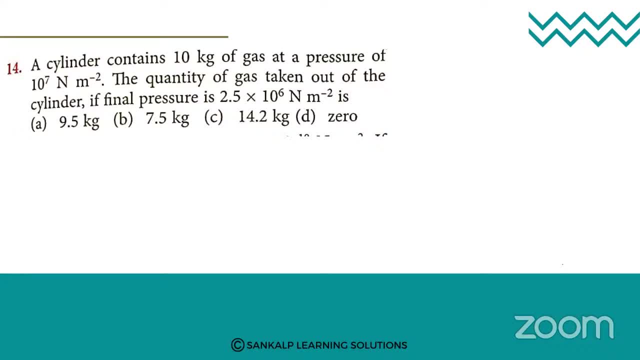 would. mass was given as 2.5 into 10 is to 6 newton per meter square. so mass, that is the first strips say we are going to use in this. so now let's look at the q-reactive Genesis. this region, main region. 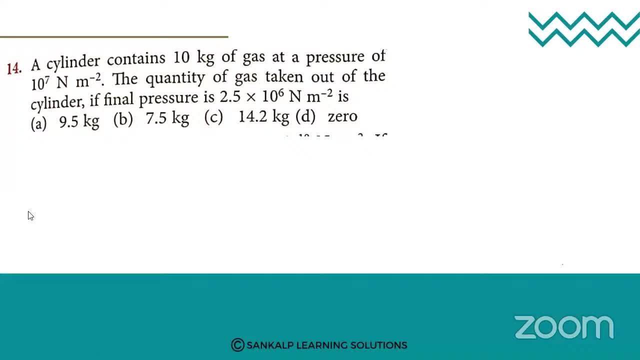 with R but max z. this by v2 is equal to m1 by m2.. So why it is? so? Because here it is given that a cylinder consists of 10 kg of gas at a pressure of- okay, the quantity of gas taken out of the 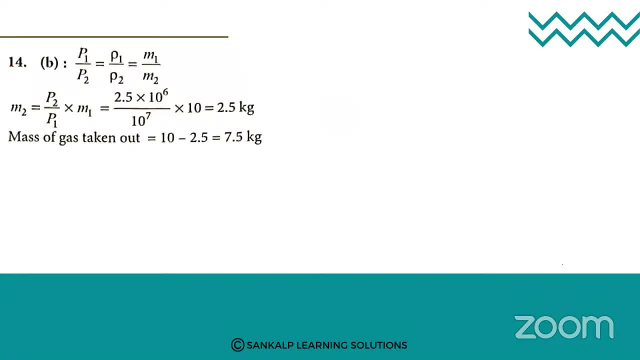 cylinder, So same density will be same. So therefore, here the volume equation we are writing in terms of density and the mass. So m2 is equal to, you know, p2 by p1 into m1. Hope so you understood this. That is, p1, v1 is equal to p2, v2.. Therefore, p1 by p2. 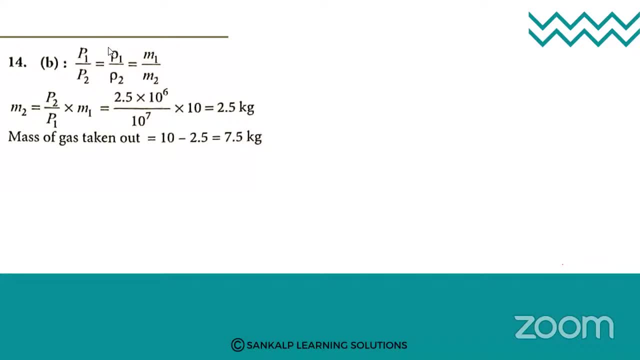 is equal to what it will be. It will be v1 divided by v2, okay, So volume term, we are replacing it with mass and the density. So therefore, as the density will be same, what will be the mass? 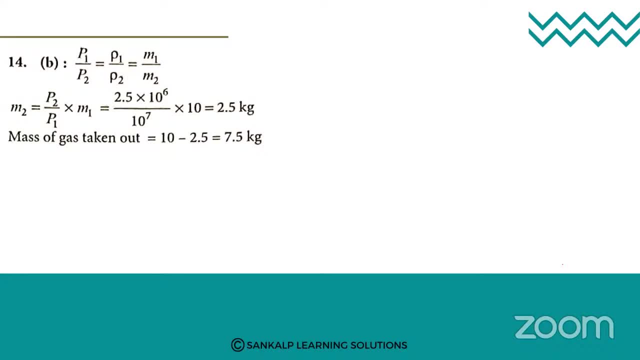 p2 by p1. into m1? It will be 2.5 kg. The mass taken out will be initial minus the final. That is 7.5 kg. is the answer C? This next question: a gas at 300 Kelvin has pressure 4 into 10 is to: 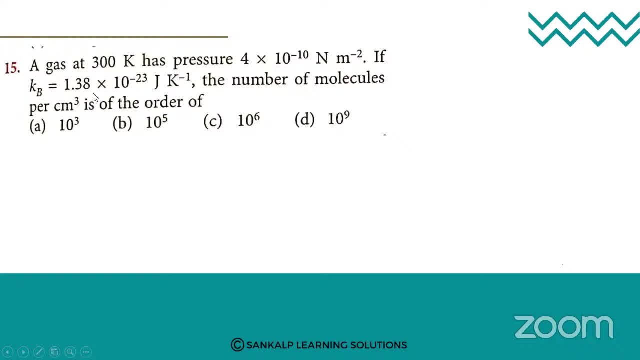 minus 10 Newton per meter square. If Kb is equal to 1.38 into 10 is to minus 23 joule per Kelvin. the number of molecules per centripetal Centimeter cube is out of the order of. So you have a gas at 300 Kelvin. It has a pressure. 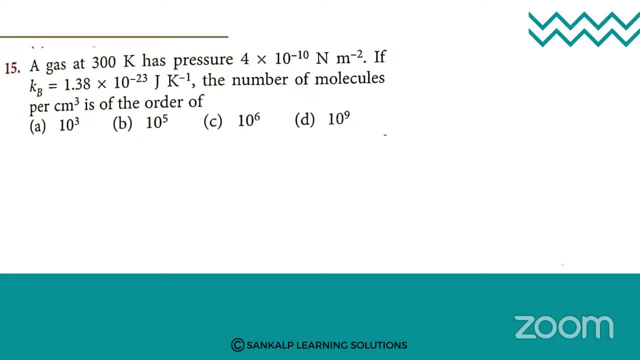 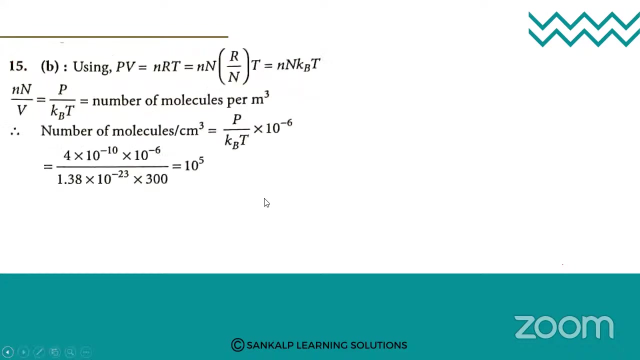 of 4 into 10 is to minus 10.. So pressure is given, Temperature is given, Boltzmann constant value is given. The number of molecules per centimeter cube is of the order of See. using PV is equal to n? rt, and here the small n can be written: Multiply and divide. 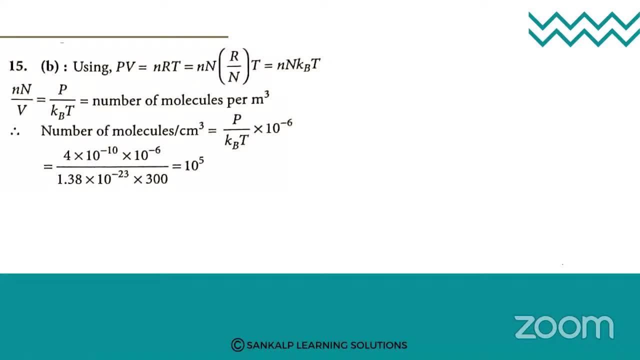 the equation by capital N, 4ardo-Mauritius. Did we get it? We did, Yes. next, N into N by V is equal to P divided by KB into T, So that is the number of molecules per meter cube. So the number of molecules per meter cube is equal to. that is P is equal. 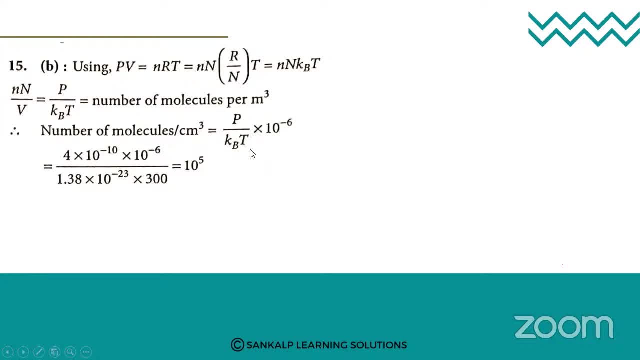 to P by KB into T into 10, raise to minus 6, because it is per centimeter cube. So per centimeter cube 10 raise to minus 2 into 10. raise to minus 2 into 10, raise to minus 2.. So that is nothing but 10 raise to minus 6.. So pressure is how much It is given as 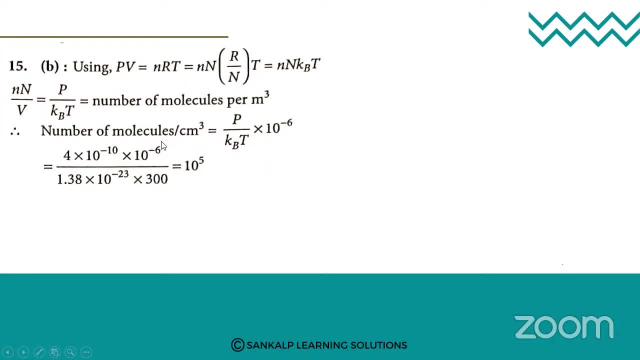 4 into 10. raise to minus 10, and here it is 10. raise to minus 6 divided by KB, the Boltzmann constant value, 1.38 into 10. raise to minus 23, into it is T temperature, that is 300.. So 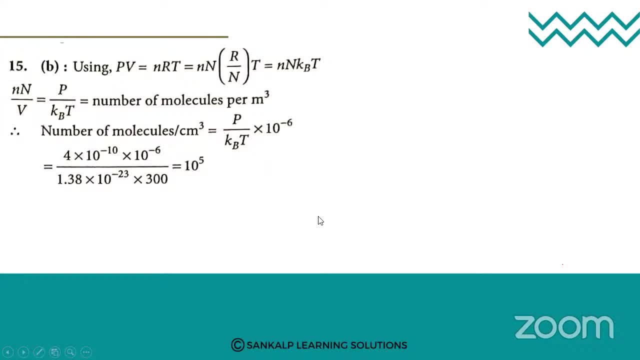 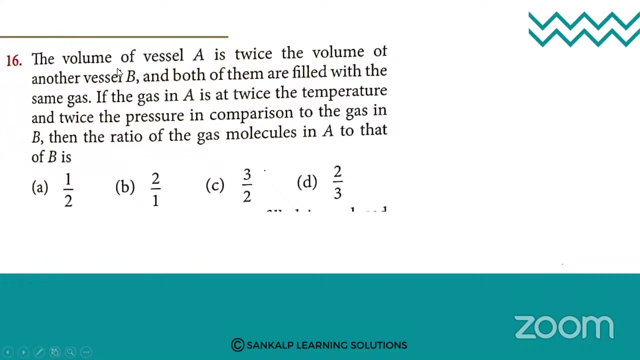 if you simplify you will get it as 10 to the power of 5.. Option B is the correct answer, Yes. next question: The vessel of the volume of vessel A is twice the volume of the another vessel B. So volume of vessel A is So A vessel volume twice that of the vessel of B, So it is twice. 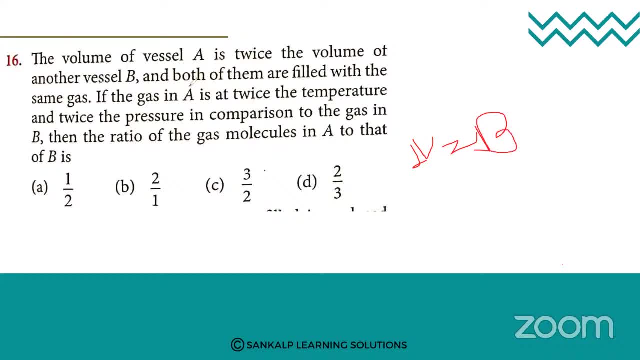 that of the vessel B here, And both of them are filled with the same gas. So both the containers are filled with the same gas but the volume is different If the gas in A is at twice the temperature and twice the pressure in comparison to the gas in B. 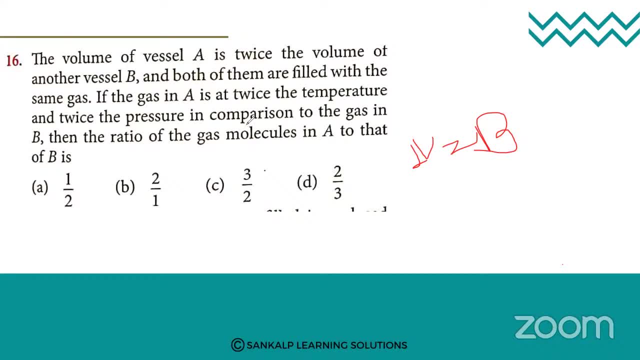 So if gas in A, its temperature is twice and the pressure is twice in comparison with the B, So okay. So what is the meaning here? compared to B, container, A vessel, only volume could be double, Temperature is also double, Pressure is also double. Okay, Then the ratio of the 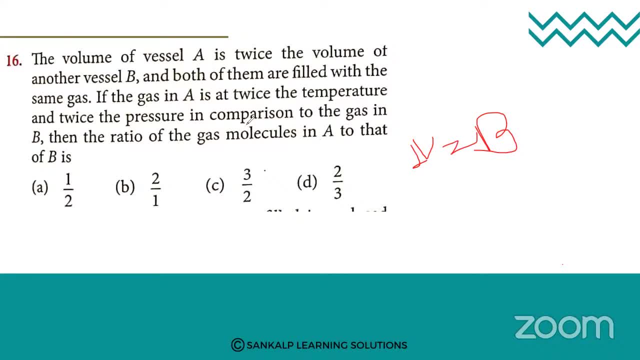 gas molecules in A to that of B is. So what we need to calculate the ratio of the gas molecules in A to that of B is. You are saying the ratio of the gas to A is the total gas. This ratio that you have given is equal to A. 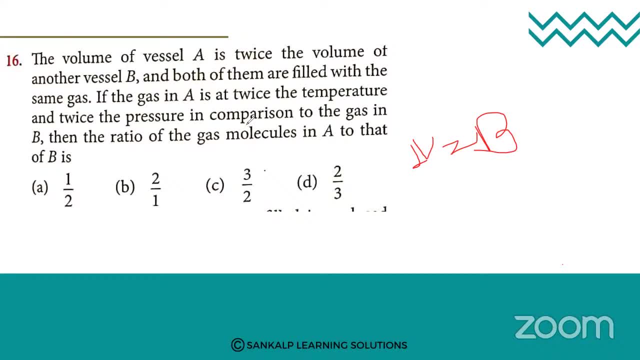 Yes, true, Okay, Woohoo. Then you can decide what is the ratio of the gas get in the vessels. A to nasty gas contains Okay, Yeah, Proprietel. whatever we were talking about is from this component, Right. 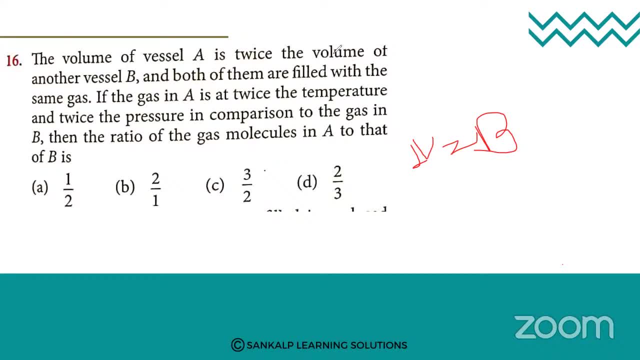 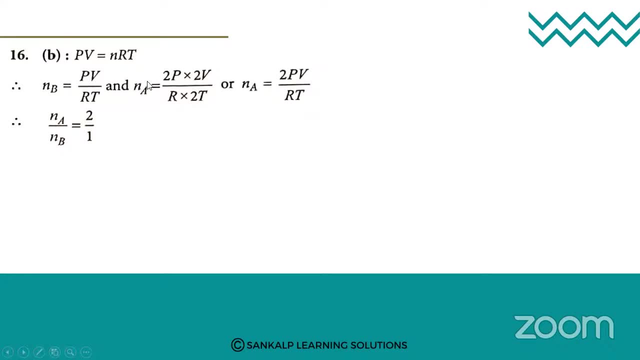 Yeah right, Parasite. Yeah, Yeah, Yeah, see here. so, as i told you, compared to a in b, in compared to b, it is everything is twice in a. so therefore, nb is equal to pv by rt for the b vessel. for the a vessel, all the values are twice. 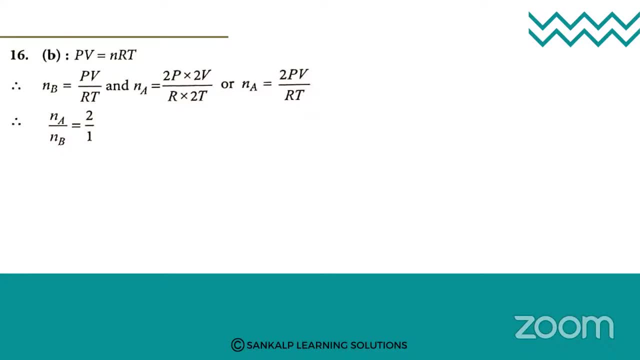 except the constant ideal gas constant. so therefore, or n a is equal to, you can generally write it as: what two pv, so two. two will get cancelled, so only the remaining is two pv divided by rt. yes, so what is pv by rt? pv by rt is nb, correct. so what we can do here? substitution cs. 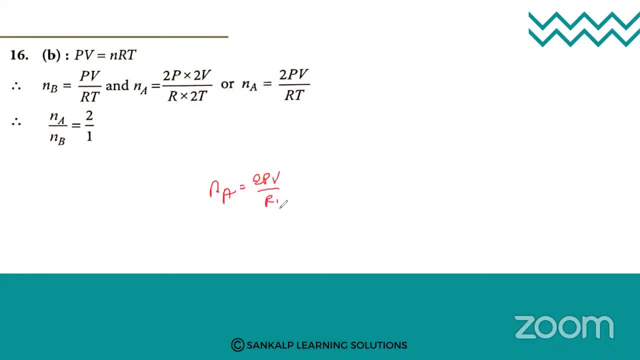 that is, na is equal to 2, pv by rt, which is equal to 2. what is pv by rt? pv by rt is nb. so therefore na by na is equal to 2 nb. or you can also write it as: na divided by nb is equal to 2 divided by 1, correct? so that is 2 is to 1 ratio. 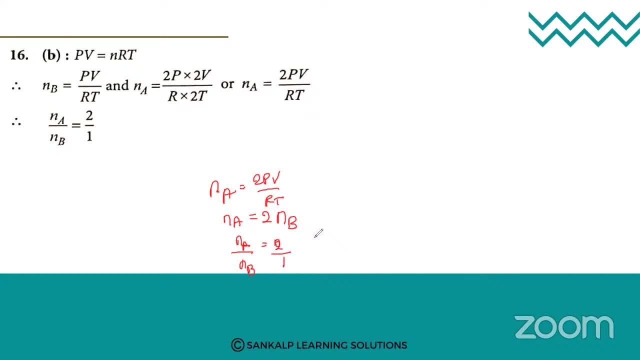 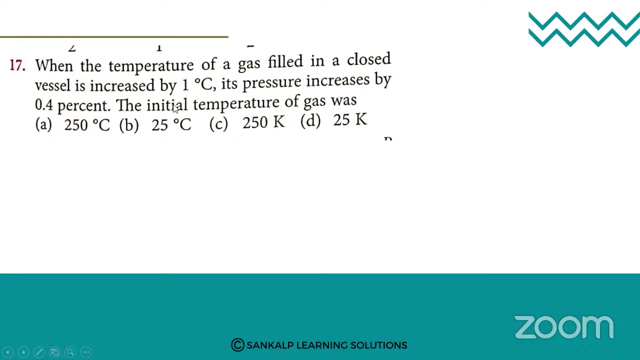 let's see the next question. when the temperature of a gas filled in a closed vessel is increased by one degree centigrade, its pressure increases by 0.4 percent. the initial temperature of the gas was: yes, when the gas of a gas, when the temperature of a gas is filled, 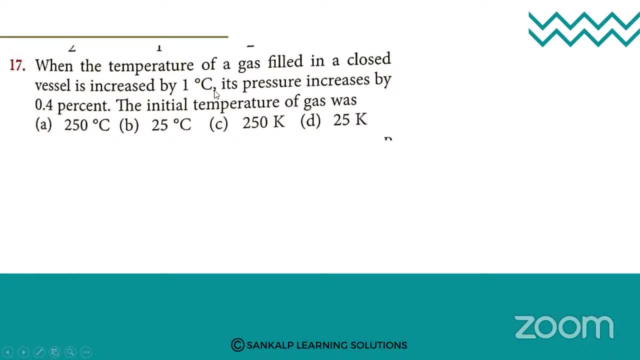 in a closed vessel is increased by one degree celsius, its pressure increases by 0.4 degree celsius, 0.4 percent initial temperature. so that is p2 by p1 is equal to t2 by t1. therefore t1 is equal to. 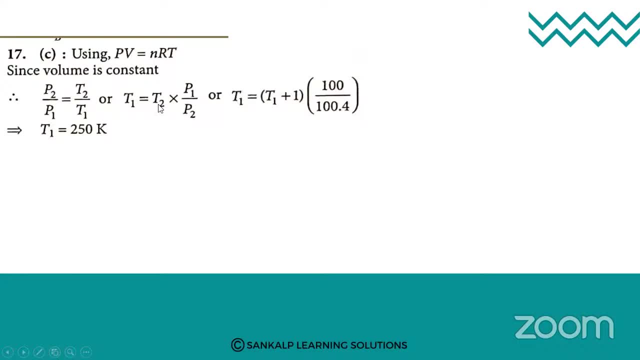 t2 into p1 by p2. so or you can substitute t2 as t1 plus 1 into bracket 100 divided by 100.4. so therefore t1 is equal to v1 by v2 is equal to v2 plus 1 into bracket 100 divided by 100.4. 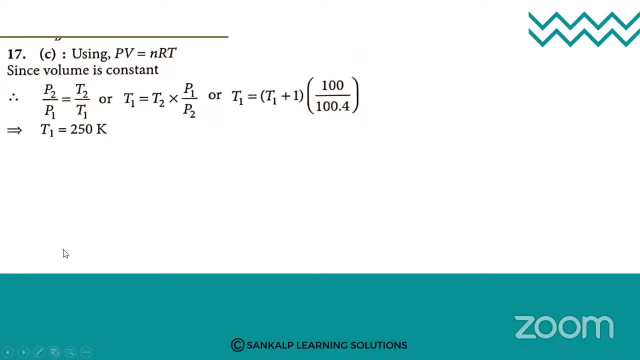 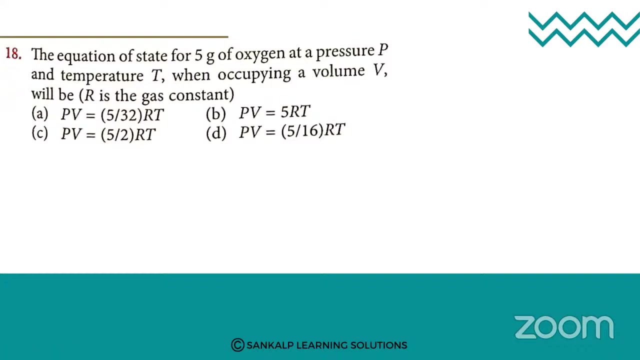 will get it as 250 Kelvin. P1 is 250 Kelvin. Yes. the next question: The equation of state for 5 gram of oxygen at a pressure P and temperature T, when occupying a volume V will be. Is the expression for PV? they are asking C. 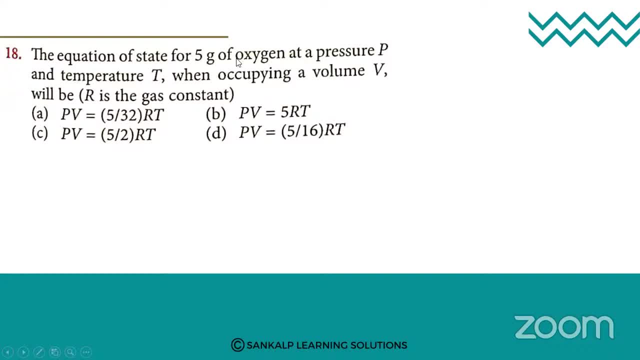 What they are saying. the equation of a state for 5 gram of oxygen at a pressure P and temperature T when occupying a volume V will be. So you can see, PV is equal to nRT or n is equal to n is nothing but m divided by molar. 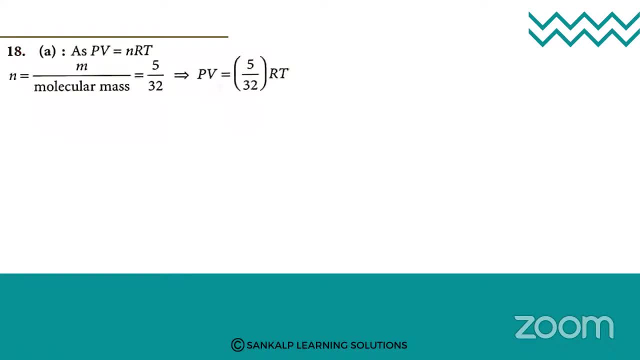 mass. So mass, how much? it is given in the question. It is given as 5 gram Molar mass for oxygen. So for the oxygen atom the molar mass is given as 32.. So therefore PV is. 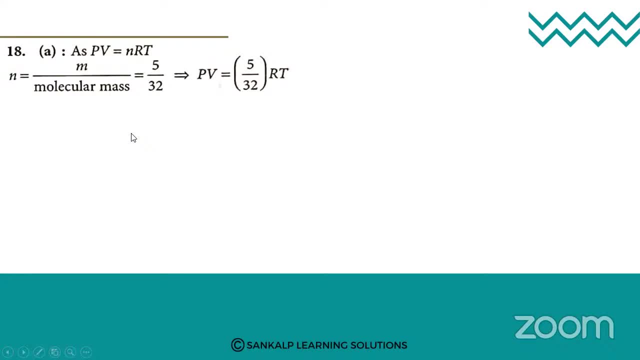 equal to 5 divided by 32 into RT. That is option A is the correct answer. So that is the answer. Let us take this question. A vessel containing 1 mole of oxygen gas and its molar mass is 32 at a temperature T, the pressure of the gas is P. An ideal vessel. 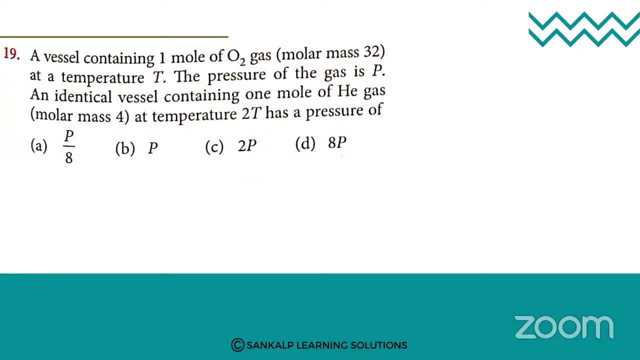 containing 1 mole of helium gas and its molar mass is 4.. At temperature 2T, the pressure of pressure C is another question. So this question: what is it So for condition? many a vessel containing 1 mole of oxygen gas, the tremors in the vessel. 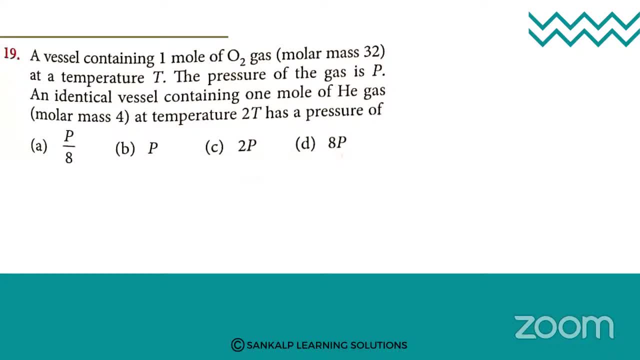 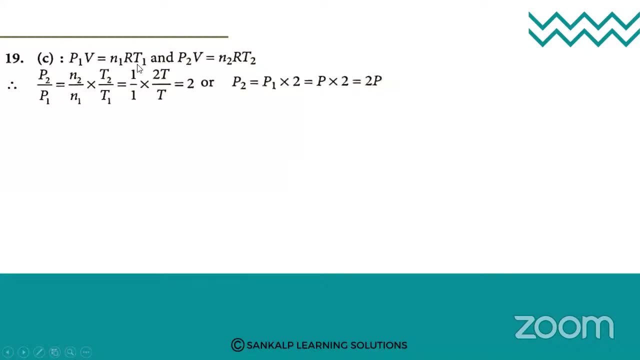 is given as 2, or the temperature of the vessel can be given as 2, or the temperature of the vessel can be given as 2.. Since this is aожу angle gas, there can be some setups that may be to be 군 the vessel from other ocean sources At current moment same. 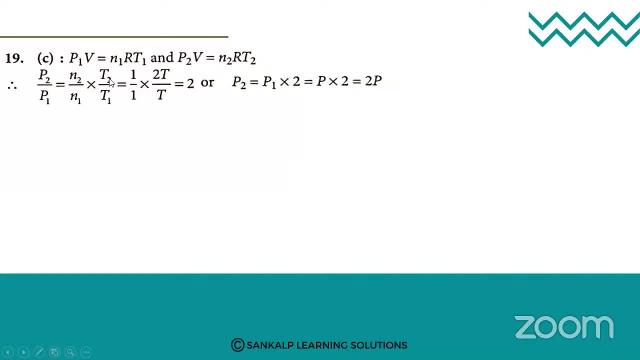 2, R, T 2 or P 2 by P 1 is equal to N 2 by N 1 into T 2 by T 1 and N 1, N 2 values are 1 and the temperature is 2, T by T, So T T will get cancelled. Therefore, P 2 by P 1 is equal. 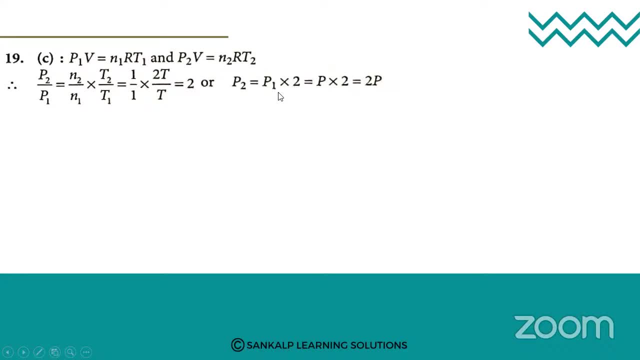 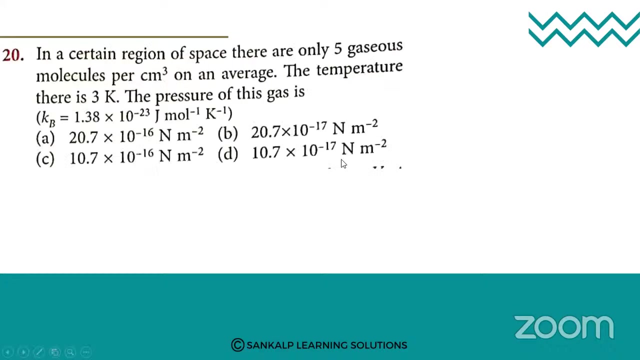 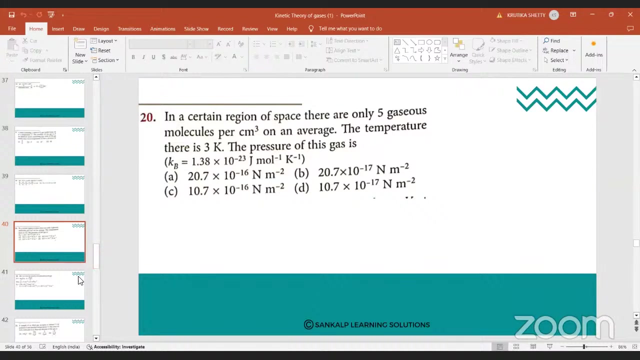 to you are getting it as 2 or P 2 is equal to 2, P 1 or P 2 is equal to 2 P, It is twice. Just take down one more question. last question: Yes see, In a certain region of free space there are only 5 gaseous molecules. 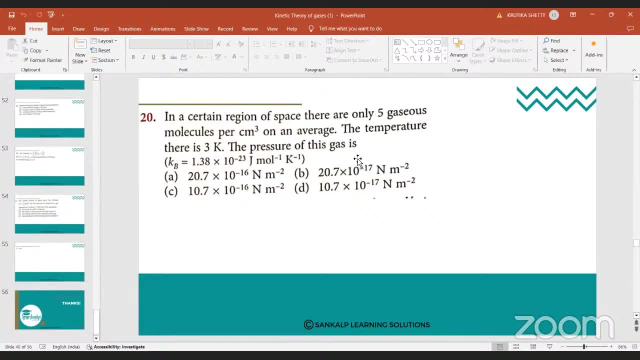 So you have only 5 gaseous molecules per centimeter cube. on an average, The temperature is 2 T per C cube. The temperature is 2 T per C cube of there is 3 Kelvin. What about the pressure? So pressure, you need to calculate N value. 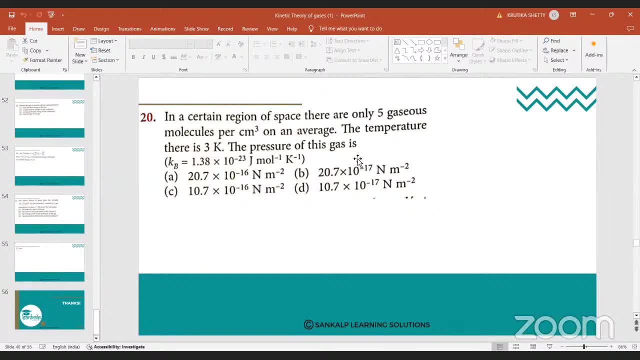 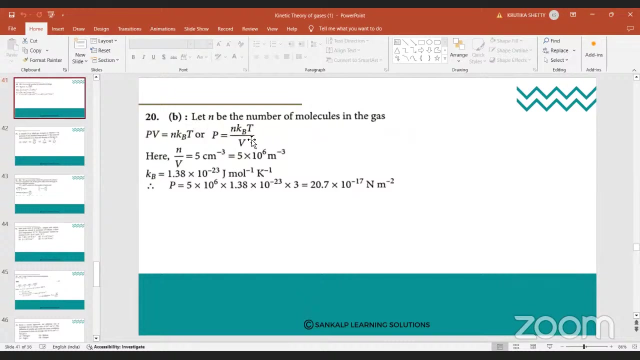 is given, temperature is given, Kb value is given. Let's see: Let n be the number of molecules in the gas. So Pb is equal to n Kb into T, or P is equal to n KBT by V. And what is N by V? N by V is 5 centimeter cube, or it is 5 into 10. raise to 6. 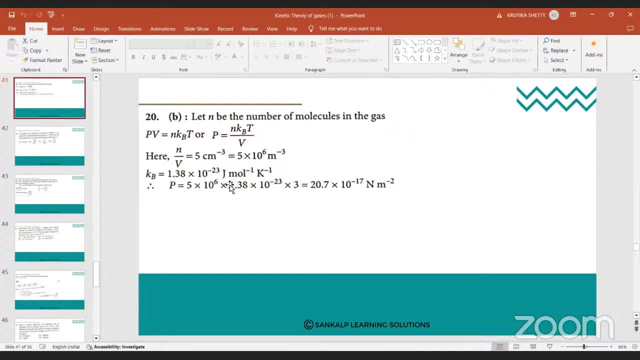 per meter cube And KB is 1.38 into 10, raise to minus 23.. So therefore the pressure will be: N by V is nothing but 5 into 10, raise to 6.. KB is 1.38 into 10, raise to minus 23, into 3.. 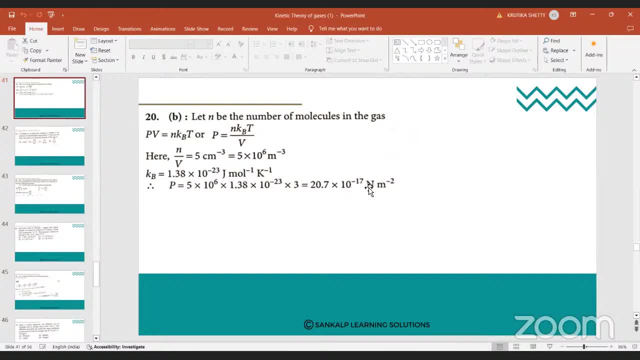 So that is 20.7 into 10. raise to minus 17 newton per meter square. Option B is the correct answer. Yes, students completed One more last question, direct question. it is C: The kinetic theory of gases gives. 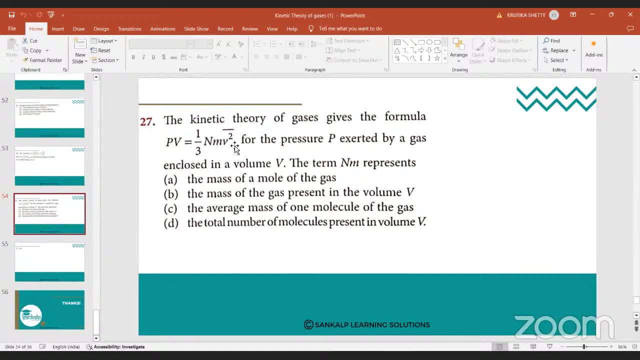 the formula PV is equal to 1 by 3 Nm average velocity square for the pressure P exerted by a gas enclosed in a volume B The term Nm represents. So in the equation you are able to see, that is, PV is equal to 1 by 3 Nm V square. So in the given equation, what is that Nm stands?